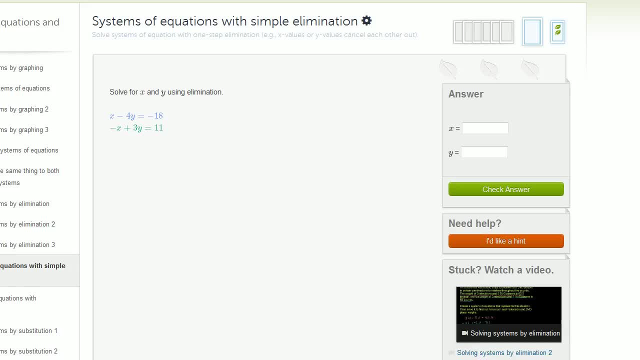 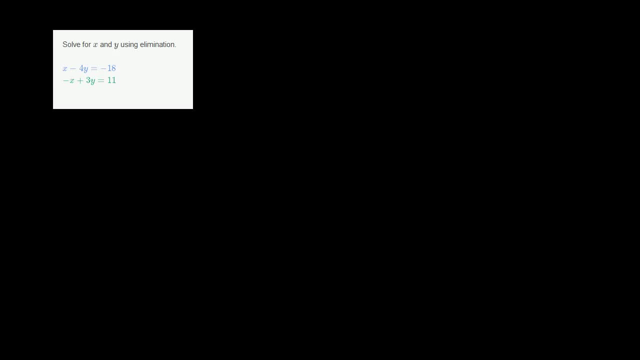 plus 3y is equal to 11.. So let's try to work this out. I'll get my little scratch pad out. This is the exact same problem. Let me just rewrite it again. It never hurts to rewrite it. get more familiarity with the problem. So x minus 4y is equal to negative 18.. And 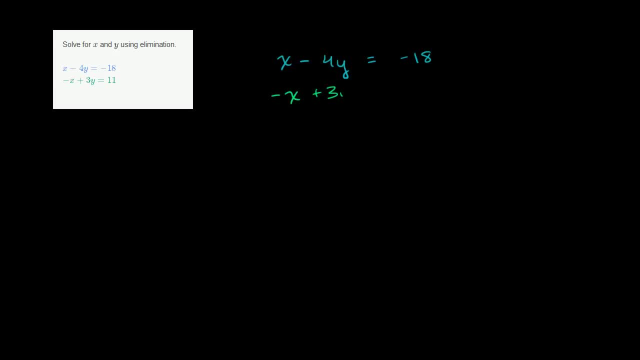 then we have negative x plus 3y is equal to 11.. So the thing that jumps out at my brain: we want to eliminate one of the variables And we have an x here and we have a negative x right over there, So that feels like those would cancel each other out very well. So. 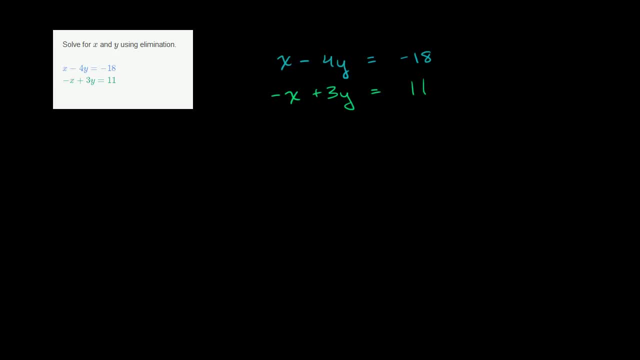 let's do that. Let's add negative x plus 3y to the left-hand side of x minus 4y, And then we can add 11 to the right-hand side because, as the second statement shows, this is equal to this. So 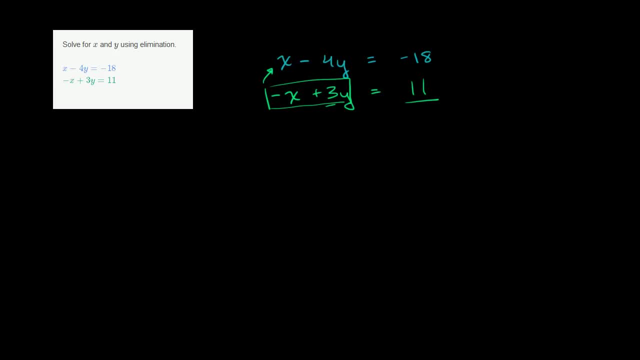 if we add this to the left-hand side, we could add the same thing to the right-hand side, But instead we're just going to add the 11, because it's the exact same thing as negative x plus 3y. So we're going to add 11 to the right-hand side. 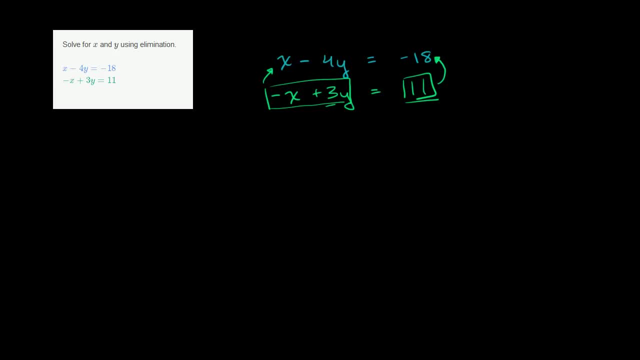 And so let's say that we have negative x plus 3y, And then we're going to add 11 to the left-hand side. Let's see what happens when we do that. Well, the whole purpose is that you have an x minus. 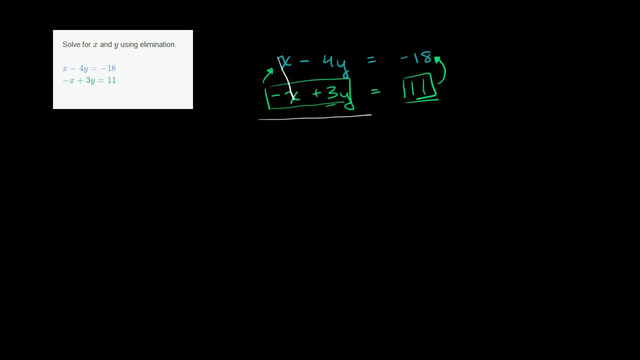 an x, Those cancel out And then you're just left with negative 4y plus 3y. Negative 4 of something plus 3 of something is you're going to have negative 1 of that something. Or you could just say negative y And then that's going to be equal to And remember. 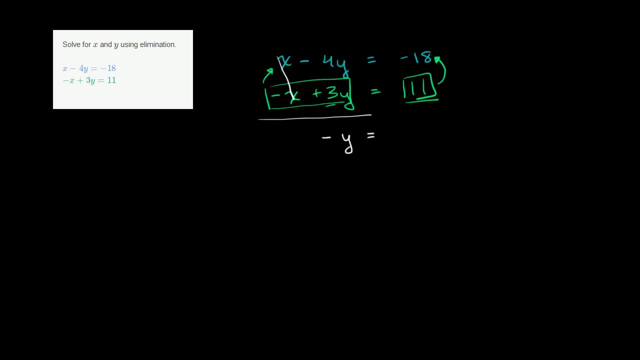 we can still say equal, because we're essentially adding the same thing to the right-hand side that we're adding to the left-hand side. 11 is the same thing as negative x plus 3y. 11 plus negative 18 is negative 7.. And now we're in the home stretch If we want to solve for 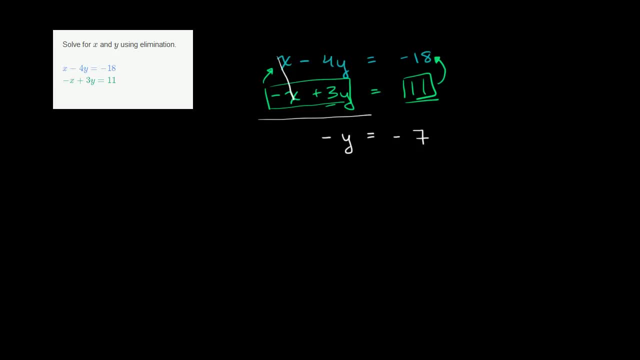 y. we can divide both sides by negative 1 or multiply both sides by negative 1, depending on how you want to view it. So let's divide both sides by a negative 1.. We are left with: y is equal to positive 7.. But we aren't done yet. We need to figure out what x is equal.